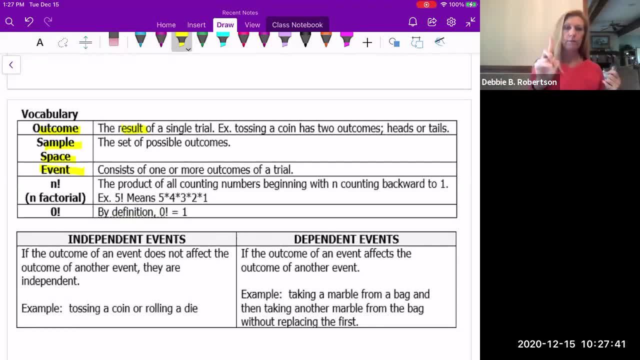 So I roll the dice once. what do I get? That's one event. I roll a dice a second time. what do I get? That's a second event. A third time would be the third event. So the event is the outcome of one or more trials. All right, n factorial. n exclamation point is read as n factorial. 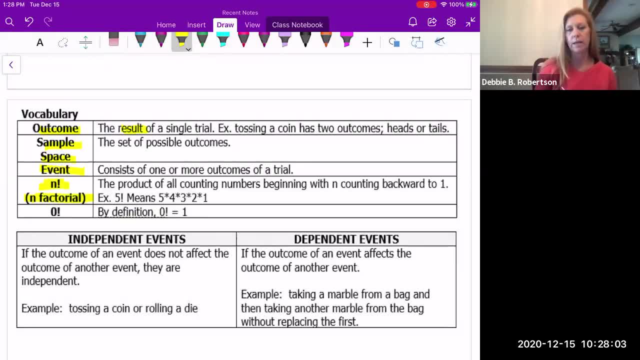 and it means whatever n is. you multiply that number, times its previous number, all the way down to one. So five factorial means five times four times three times two times one. Okay, zero factorial by definition is always going to be one. Now we have to also. 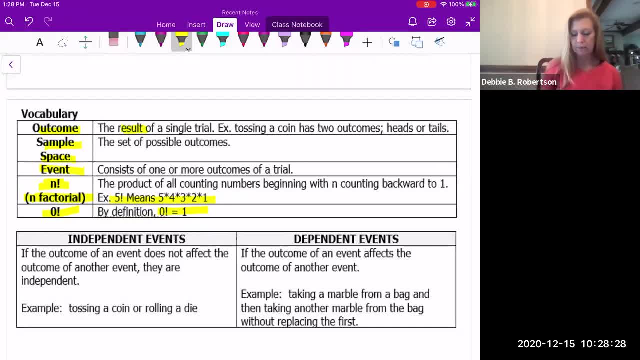 understand the difference between independent events and dependent events. Independent events: an outcome does not, it's not affected by the outcome of another event. All right, and a really good example is if I toss a coin once and I get a heads or tails, all right, and then I toss it again, I could still get a heads or tails. The first toss had no effect. 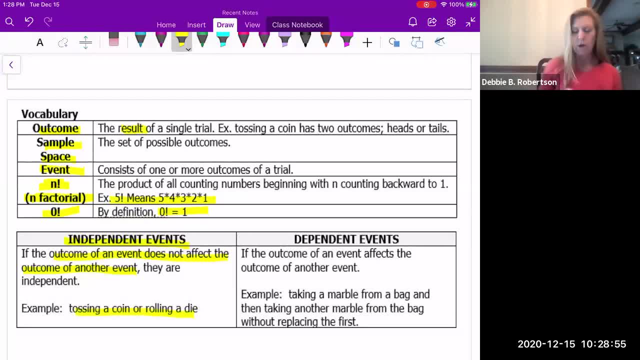 on the second toss and the same thing with rolling a die. However, dependent events, all right. the outcome of an event does affect the outcome of another event. So an example here: I have a bag of marbles. Maybe I have 10 marbles in the bag and I take one out. 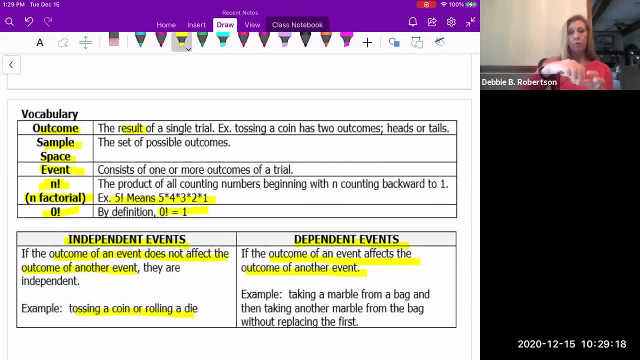 If I don't put that marble back in and I go to pick another one, I have one less okay chance of picking a particular marble than I did when I had the 10 in there. So the taking the marble out of a bag, then taking another without replacing the first one, of course, a. 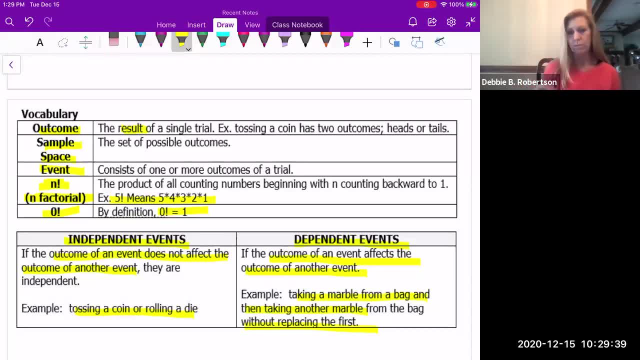 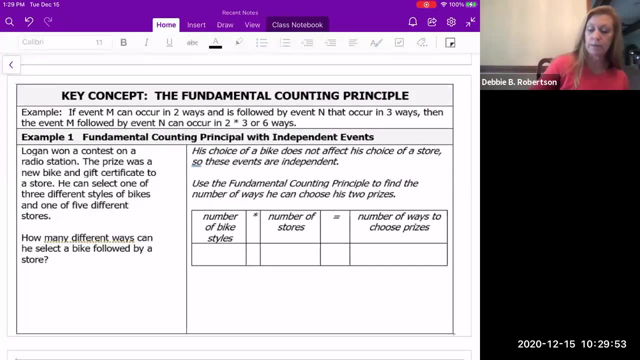 I replace, all bets are off. Okay, it would become independent. but without replacing, then it's dependent. All right. key concept here is our fundamental counting principle, and you probably addressed this in middle school. All right, I have simplified this because I think representing it with numbers is just a little bit more complicated. I'm going to go ahead and do that. 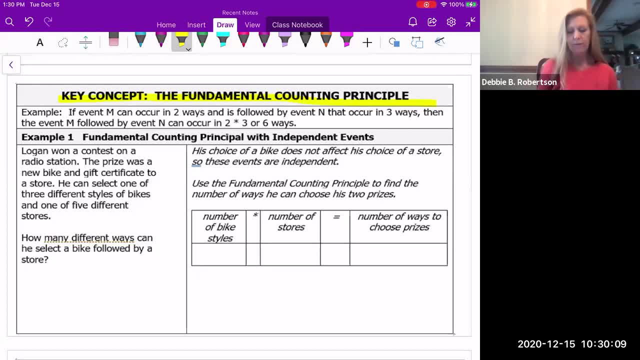 I'm going to break up structured characters and so on and so on. So I'm not going to go through my simple bringenism, I'm just going to go all through. So one of the first inputs is four ways SSD. So in here m is the four smashed or kilo. 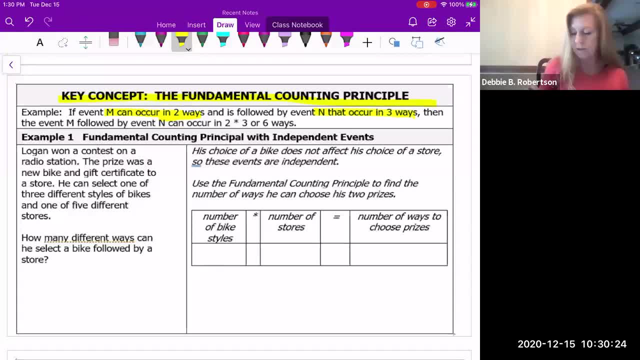 or V, moral, equal or other variable, because m actually represents the parameter of m, And so we've all done that so far to just make sure that you've all got that in front of you. And so I'm just going to- I'm going to have a little bit of木, rather, but 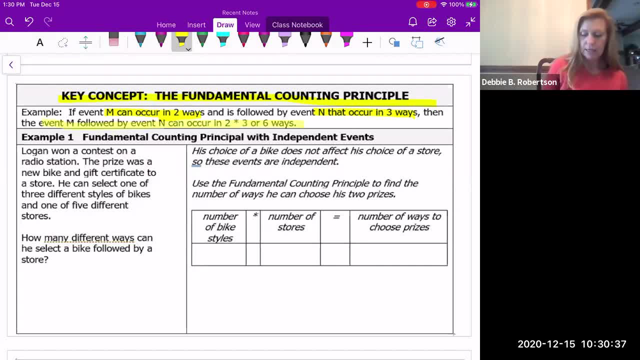 let me not go there on the edge. I mean that's a little complicated. event n can occur in two times, three or six ways. So the fundamental accounting or counting principle- not accounting, all right, takes that m events. how many ways can that occur? 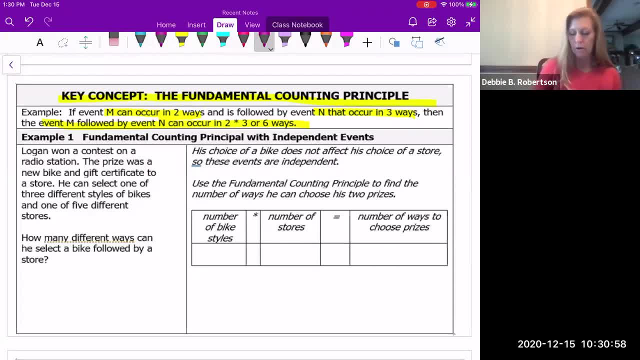 and how many ways can n occur, all right, and multiplies them together. So I have m times n, And I put it with lower case variables because they're representing how many ways m can occur and how many ways n can occur, All right. so in this example here, Logan won a contest on a radio. 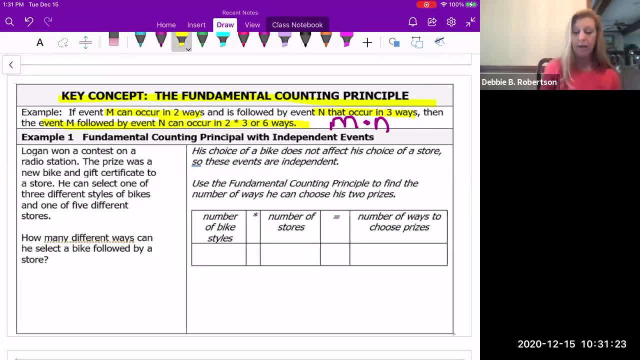 station. The prize was a new bike and a gift certificate to a store. He can select one of three different styles of bikes. all right, so three different types of bikes and one of five different stores. I wish I was Logan. Logan, I wonder if you really did win. 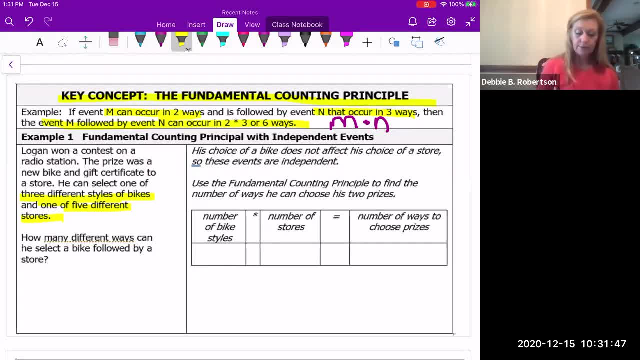 this prize? All right, how many different ways could he select the bike, followed by selecting the store he's going to use the gift certificate at, Since his choice of selecting the bike is not affected by his choice of what store he gets his gift certificate? 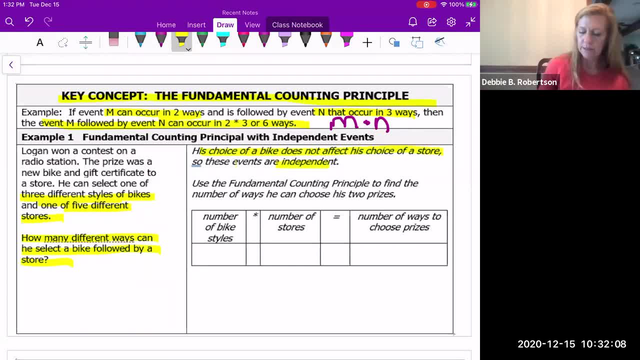 from not affected, then the events are independent. Now we're going to use the fundamental counting principle to see how many different ways he could win his prize. All right, so he has three different choices of the bike and he has five choices of stores. 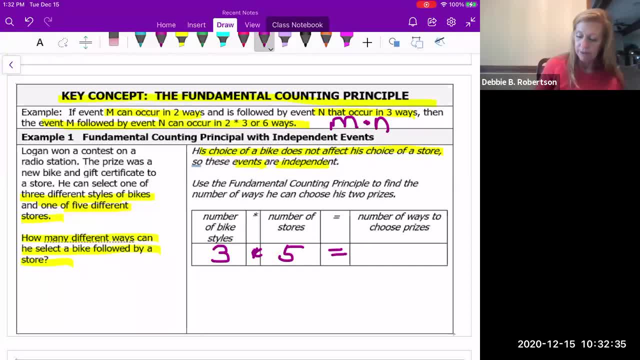 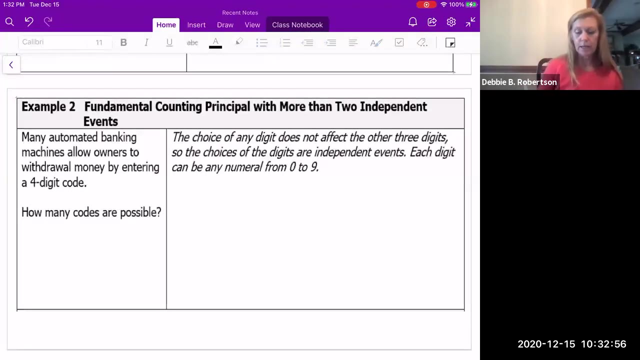 So if I multiply them together, there are 15 different combinations ways he could choose his prize or receive his prize. okay, Yeah, I'm not seeing any chats right now. All right, in this next example, again, we're using the fundamental counting principle, but this time with more than two. 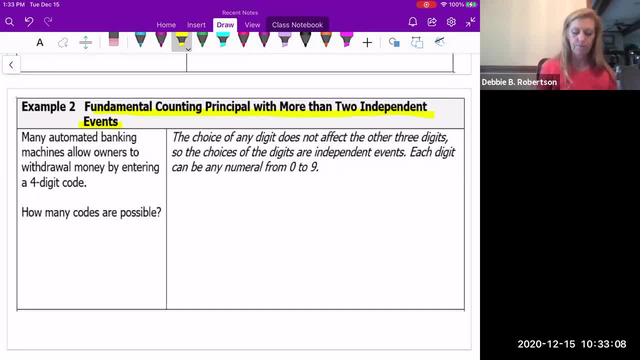 independent events. Still independent, but more than two. So here's the example. Many automated banking machines allow owners to withdraw money by entering a four-digit code, Like when you. I guess when you go to the ATM, though, you have your card, So I don't know if you have to put in. 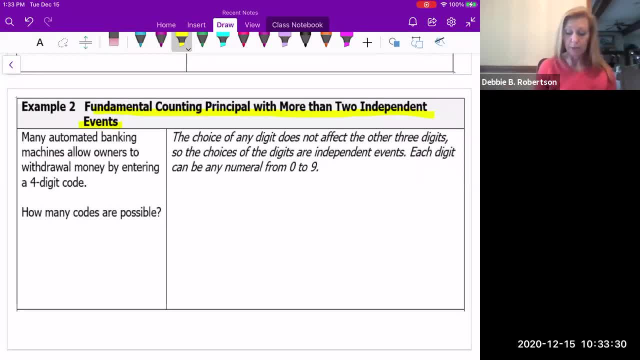 a code or not. To be honest with you, I don't have a debit card, so I don't go to the ATM machine, But anyway. so we have a four-digit code and we want to know how many codes are possible. 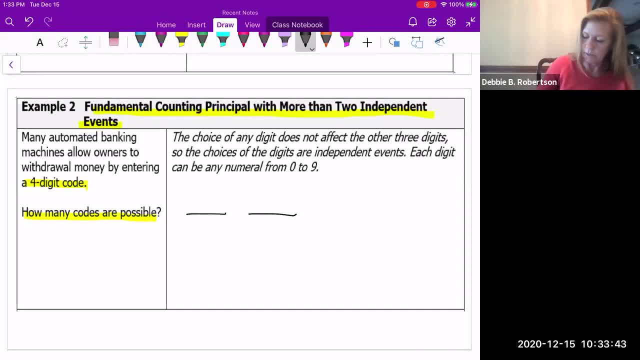 So, again, I have a one, two, three, four-digit code I need to come up with, And there are zero. each digit would be from zero to nine. Okay, So, Chris, how many numbers are there from zero to nine? 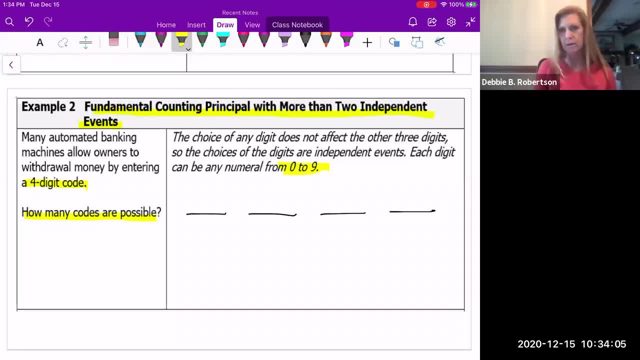 Just, I'm only looking at zero to nine. How many numbers is that, Chris? are you with us? Connor, can you help us out here? Are you counting the zero as well, Because then it would be nine? I am counting the zero. 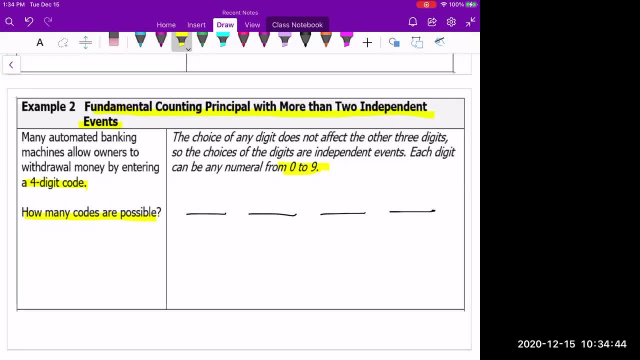 Oh then 10.. Yes, that's what we're looking for. So any particular number- all right, N can be- is going to be 10 here, right, There's 10 different possibilities if I'm choosing a digit from zero to nine. So my first digit in my code. 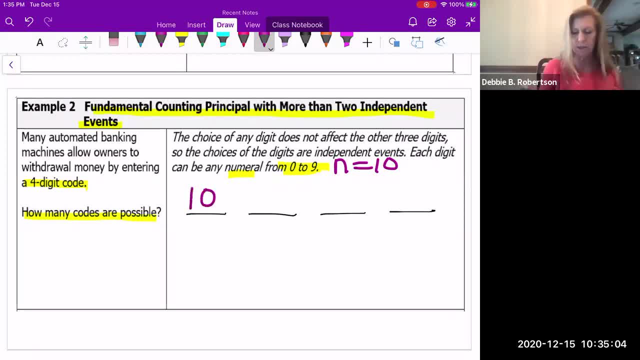 being N, I'm going to be 10.. So I'm going to be 10.. So I'm going to be 10.. So I'm going to be 10.. Anywhere from zero to nine has 10 possibilities. Well, each of those digits, I can choose a number between zero and nine. It's okay if I already used 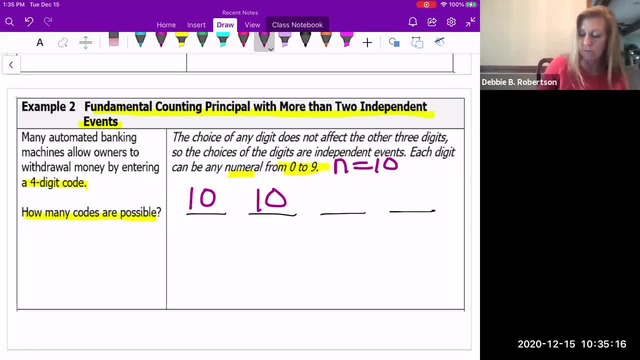 it on the digit before. So that means, for each of these I have 10 possibilities of choosing. whichever digit I choose, from zero to nine, And to determine how many different codes I could have, I'm going to multiply all these together. So how many codes in all will I have? Jack Kane. 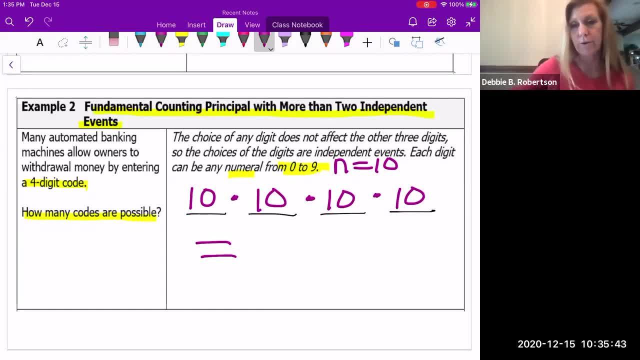 Can you repeat the question: How many codes in total could I possibly have? It would be 10,000. Exactly, So I would have 10,000 possible codes, All right, So notice what we did in both examples. In the example above. 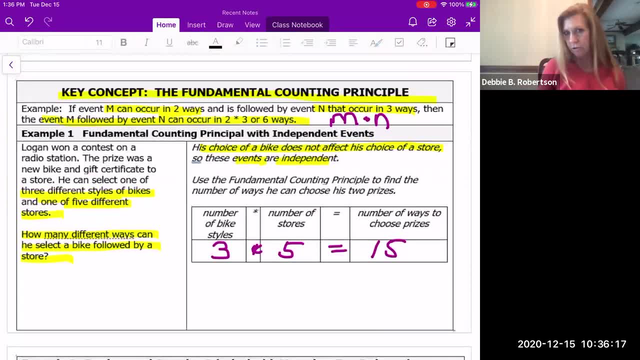 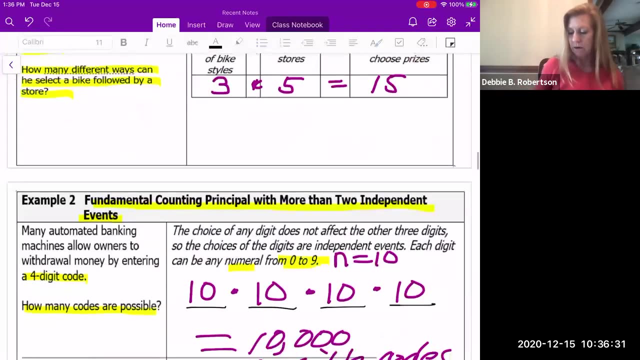 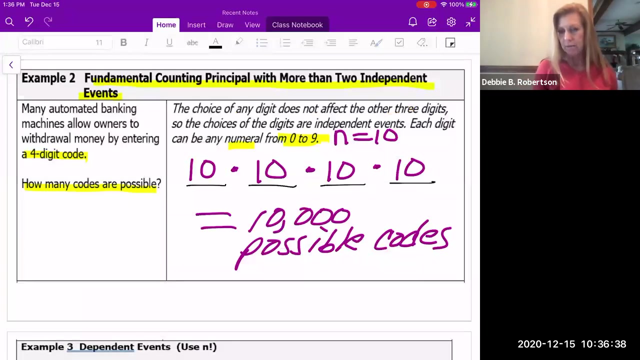 we had three bikes to choose from and five stores to choose from. They were independent of each other as far as what got chosen, which meant there were 15 combinations we could have. And then here we had to choose a four-digit code, but each one of those digits had 10 possibilities. 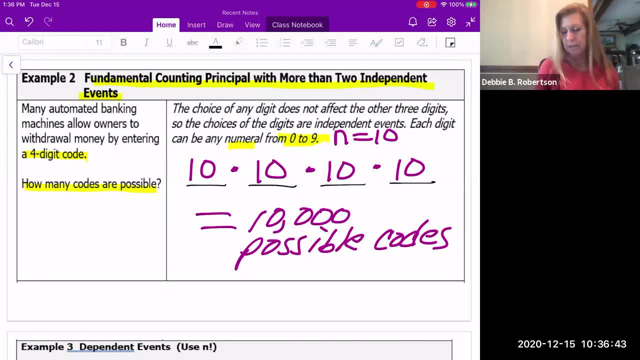 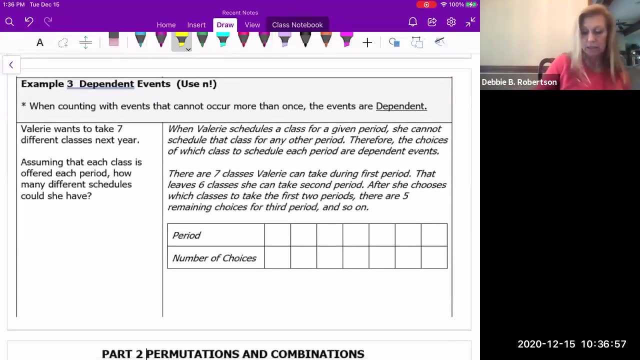 So we multiply that 10 times, 10 times, 10 times 10, and we ended up with 10,000 possible codes. Okay, All right. Let's look at dependent events And notice. I'm giving you a little bit of preview here. 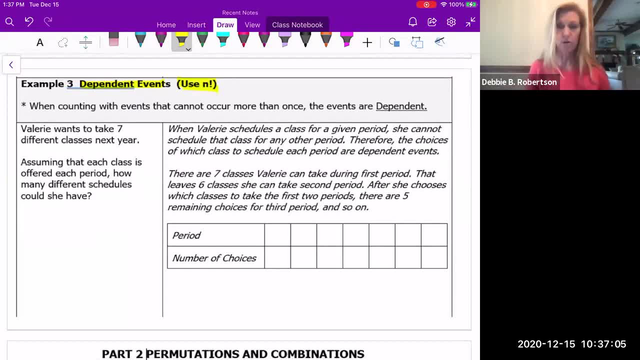 And that when we have dependent events and we're using the fundamental counting principle, we're going to use N factorial, but we're going to see how that works. So when we're counting with events that cannot, events that cannot occur more than once, 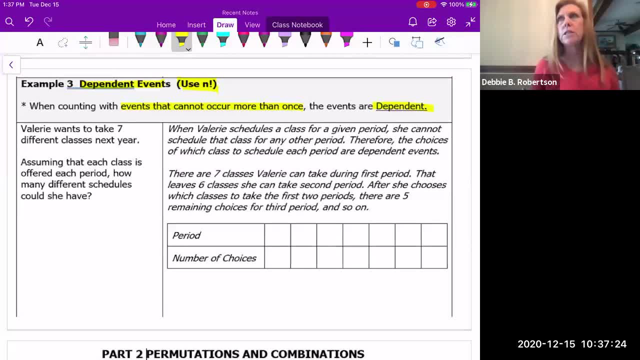 the events are dependent. So let's just say that I have a deck of cards and I pick a card out. If I get the queen of hearts and I don't put it back in the deck, well, I can't get. pick another card and get the queen of hearts again. 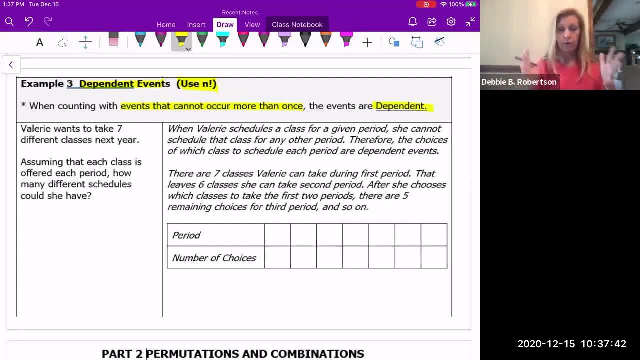 So my 52 cards the first time I picked that card. the next time I go to pick, I only have 51 possibilities, right, Okay? So in this example, Valerie wants to take seven different classes, seven classes next year. 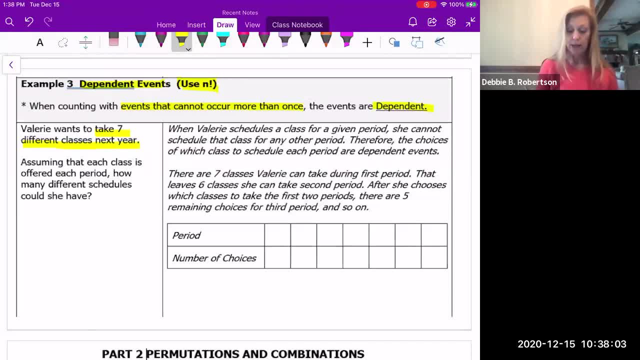 assuming that each class is offered each period, how many different schedules could she have? So that means I have seven periods. I'm going to take a class. So in my I'm making myself a chart and I know I've got seven periods. 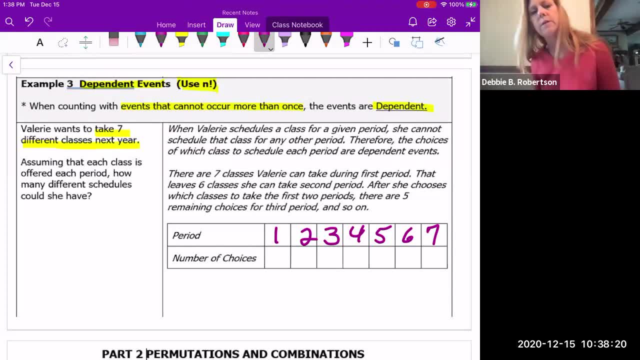 I need to schedule for makes sense. You guys do that all the time. You just don't get a choice in what you take first. Sometimes in college you can get a little bit lucky and choose when you take your classes- Not so much as freshmen, though. 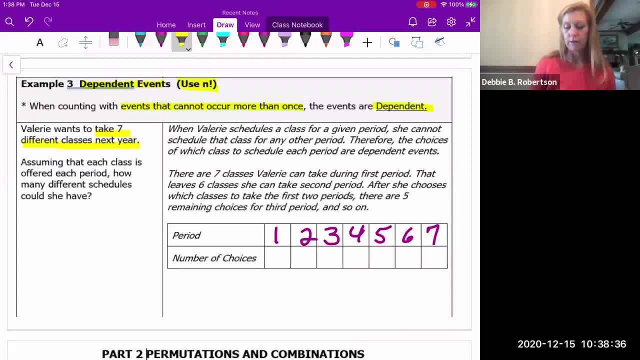 All right. So when she schedules a class for a given period, she cannot schedule a class for any other period. Therefore, the choices on which to schedule the class are dependent events. All right, Because once she chooses, once she selects biology- let's say, maybe she does that for first block- then biology is out of the picture and she only has six other subjects to choose from. 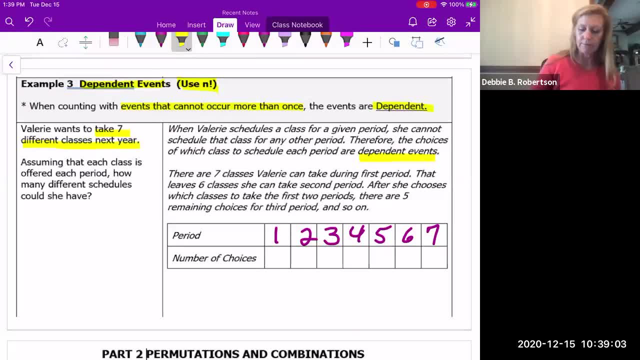 So her first block. she has seven possibilities that she could end up choosing, But then, once she chooses that one for first block or first period, then she only has six classes left to choose from. on her second belt, Now that she's chosen two blocks, that takes another away. 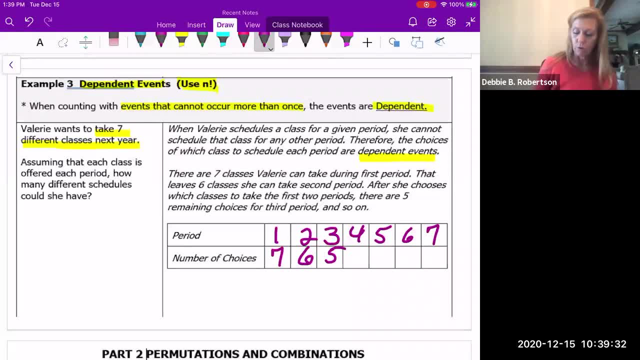 So third block, she only has one. So third block, she only has one. So fourth block, she only has five to choose from, and fourth four to choose from, and fifth block three to choose from, and sixth block two to choose from, and seventh block is whatever was left. 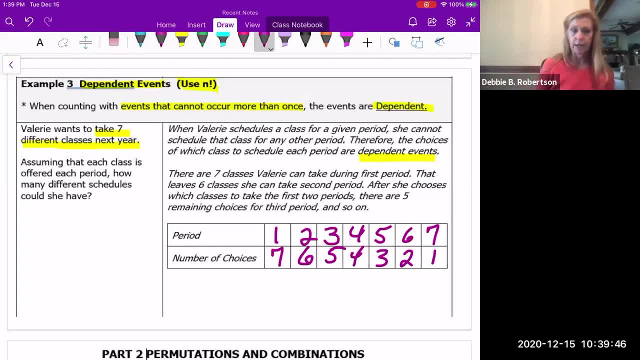 So that's how many choices she has, each block All right. But we want to also know how many different schedules could she have? So I'm using the fundamental counting, So I'm going to say my different choices, or my number of schedules would be seven times, six times, five times, four times, three times, two times one. 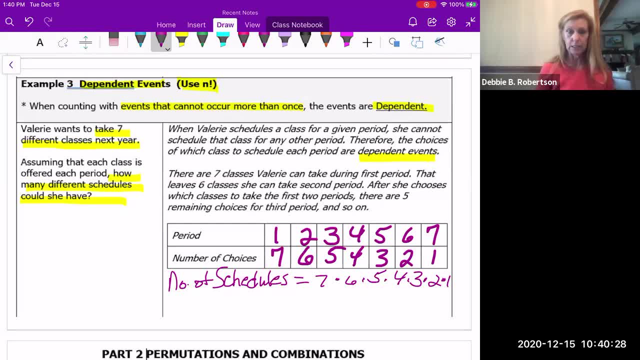 Now sometimes that gets really tedious. I don't care if you're even typing It into the calculator, It's still like really this times this and this times this gets crazy. So we can rewrite this as seven factorial. Now can I get someone to put seven factorial into Desmos and tell me what that value is? 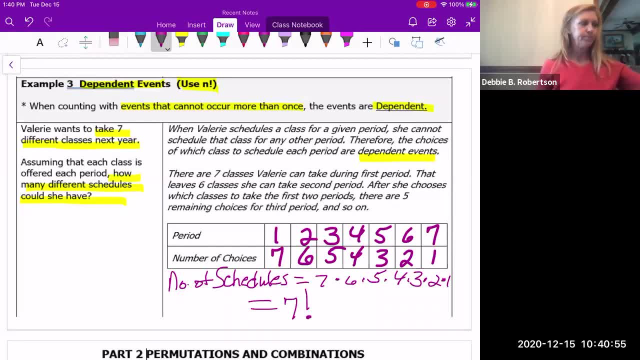 And if you have it, please raise your hand. Breeden, I saw your hand up. Can you tell me how much or how many different schedules she could have? 5,040.. Nice, And if anybody did not get that literally in Desmos. 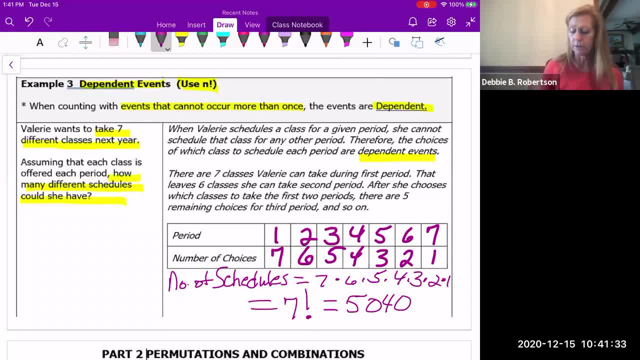 you're going to have to go to Desmoscom. Just type seven and the exclamation point and you're good, All right. So 5,040 different schedules- All right. Seems kind of crazy, huh. Imagine poor Dr Judge having to create all of the schedules for you guys every year. 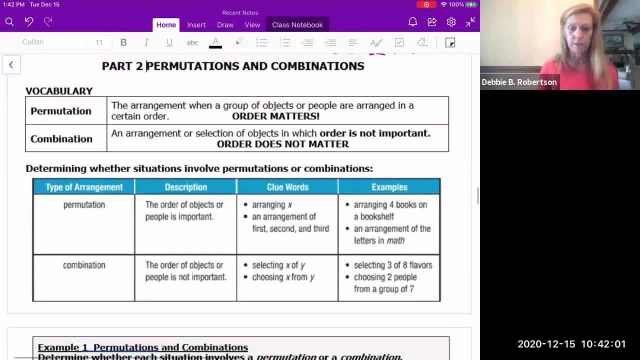 All the students. It's a lot to deal with And it's a lot more than seven different classes or subjects. All right, So our part two of this is permutations and combinations. In a permutation, that's when we're taking a certain set of objects. 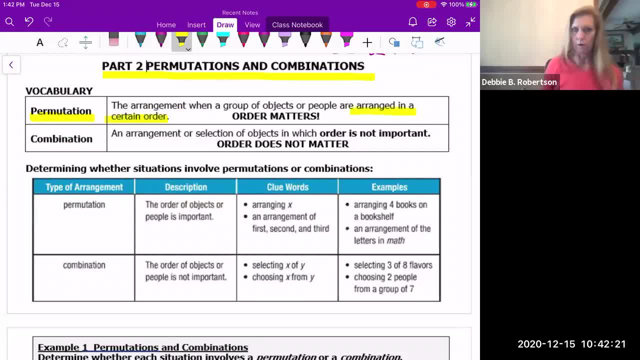 and we're going to arrange them in a certain order. All right, Kind of like Monica on Friends. Everything has to be in its place. All right, Order matters. It's huge for a permutation. That's what a permutation is about. 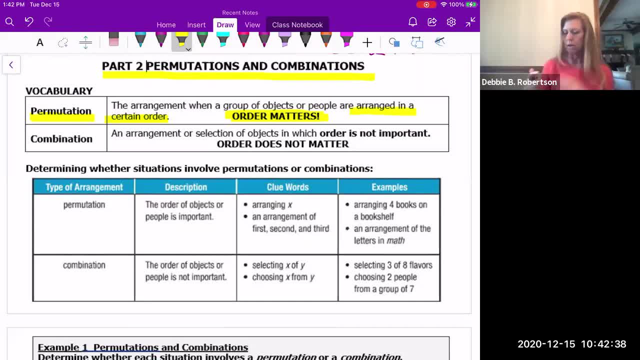 I'm picking things, but I'm picking them in a particular order With combinations. then we're just picking, All right. It's like, okay, there's 10 options for you, And I'm like you know what, I just don't care. 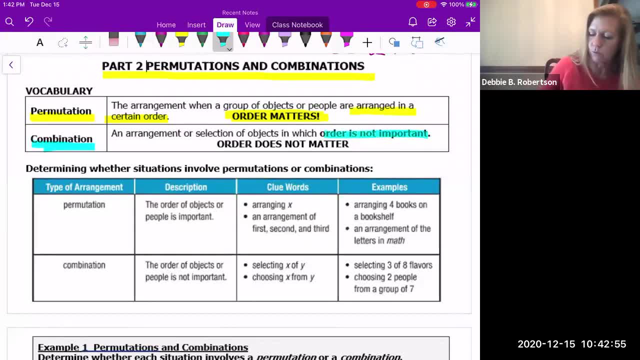 Just give me three, All right. So order is not important, It does not matter, That is important, It's a combination, All right, And kind of a good word. there is selection. I mean, they might say in a permutation that you're selecting for this. 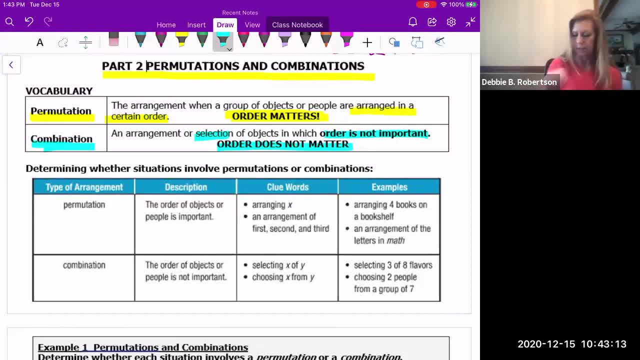 but you're looking to see, like what is it you're talking about? Does order matter? So down below here there's some. this is a really good chart to help you understand, All right, When to use permutations and combinations. So you really should make a point of this chart. 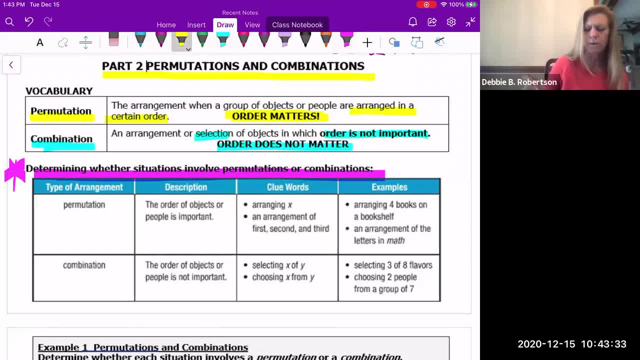 Because that's probably the hardest part in this lesson- is which one am I going to use? And they don't tell you always. So again for the permutation, remember that order matters. All right, So we might be arranging X, All right. 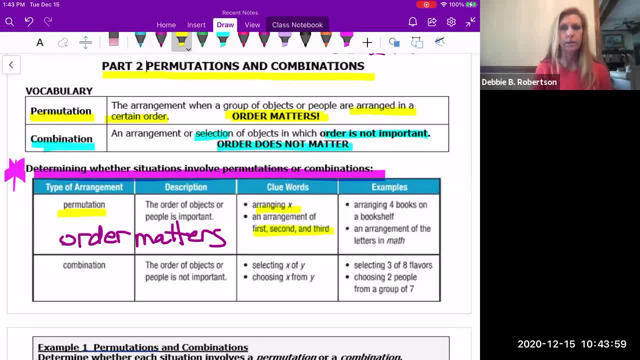 A good example is what's going to come First, second or third. Maybe it's a first place winner, second place winner, third place winner, that kind of thing. Maybe I'm going to arrange books on a bookshelf. 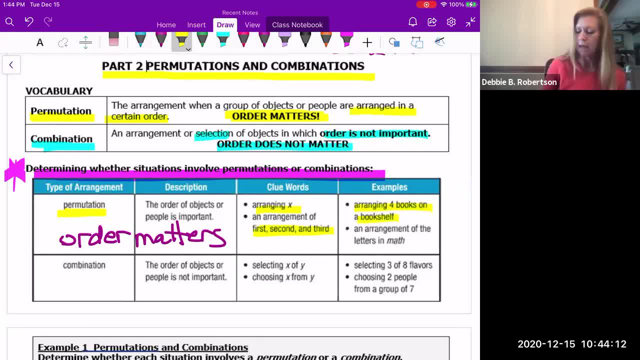 And of course order would matter to me. if I'm going to do that, Maybe the arrangement of the letters in the word math. Well, if I rearrange the letters then I'm not going to get the word math. So order is going to matter there. 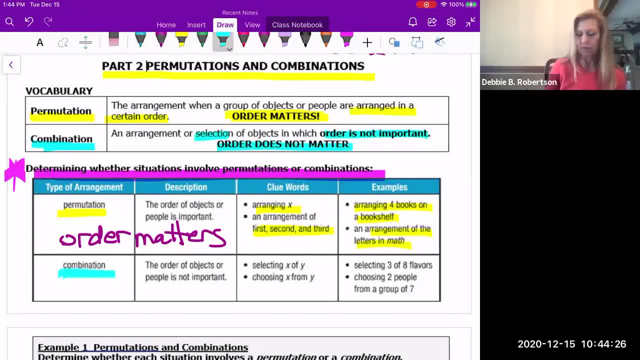 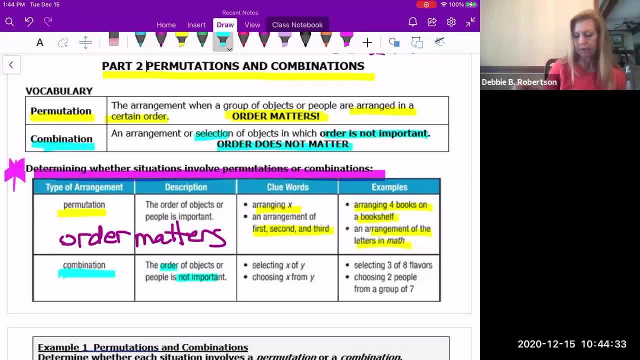 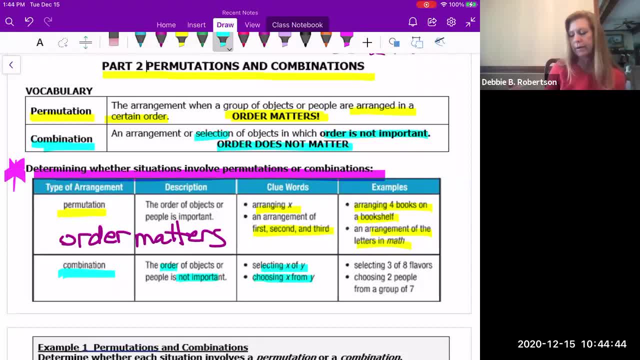 All right. Another way to phrase it is choosing X out of Y. All right, And here's an example. I'm going to select three out of eight flavors at the ice cream store because I'm going to get a triple scoop. of course you know if you've ever seen me eat ice cream. 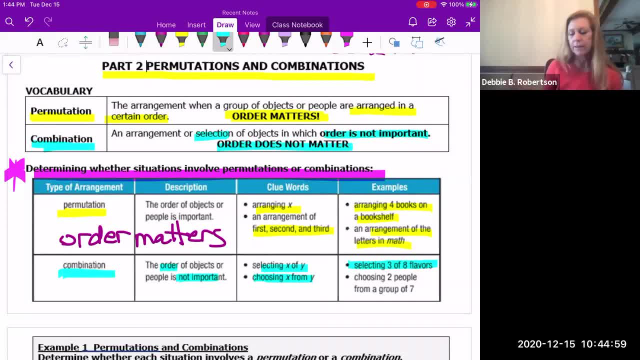 And I don't care which one you put on, the bottom and the middle And the top, just I want these three. or give me three, All right, Or choosing two people from a group of seven. you know, maybe I have seven people in my. 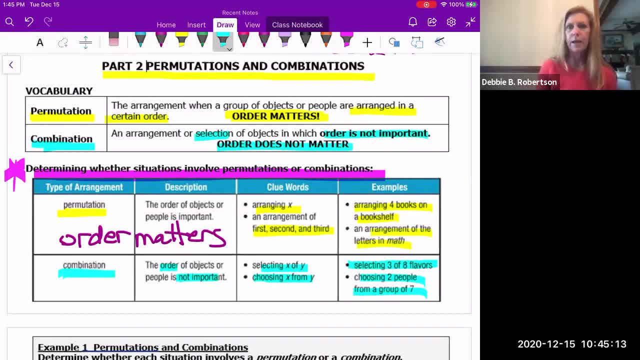 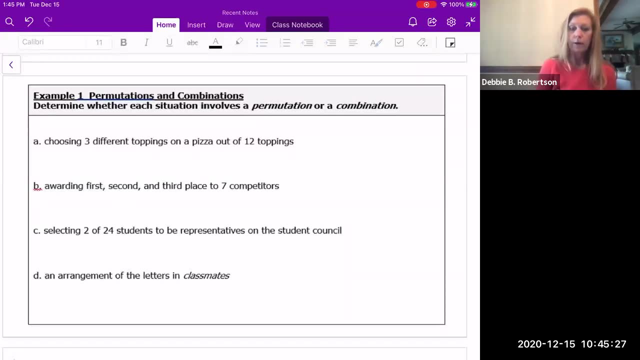 room during one lunch And I need a couple to help me carry some books, So I'm just going to grab two. All right, So that's a combination. So now that we've done that, I will end up calling on you. 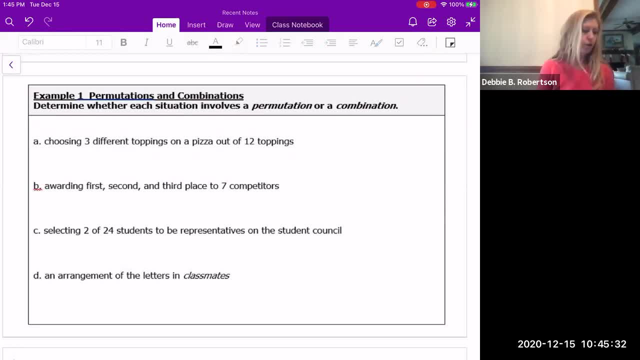 Tell me If this scenario represents a permutation or a combination, Aralise, choosing three different toppings on a pizza out of 12 toppings? permutation or combination, Aralise? are you with us? All right, What about Georgia? A combination: 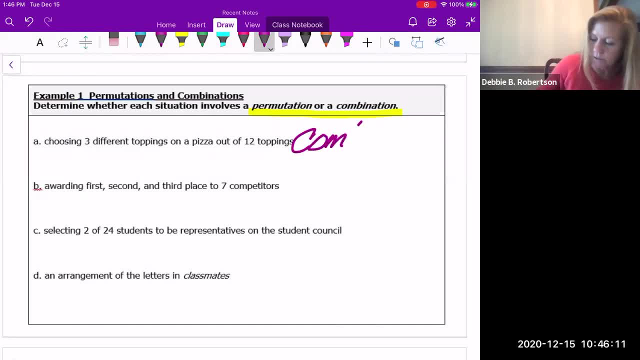 A combination. Good, Because the order doesn't matter, I just want those three toppings on my pizza. All right, What about awarding first, second and third place to seven competitors? Logan, Logan, let's see if you can earn that bicycle and that gift certificate. 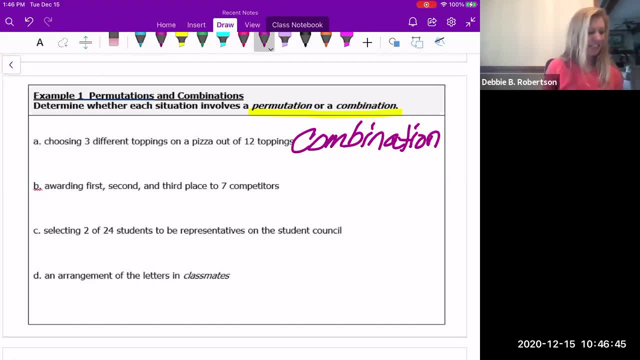 Are you with us? All right, Madison? Permutation: Yes, because I'm doing an order here for second and third. So it's a permutation. Okay, Permutation Good. This seems very basic, but we have to be able to figure that part out before we can do the next. 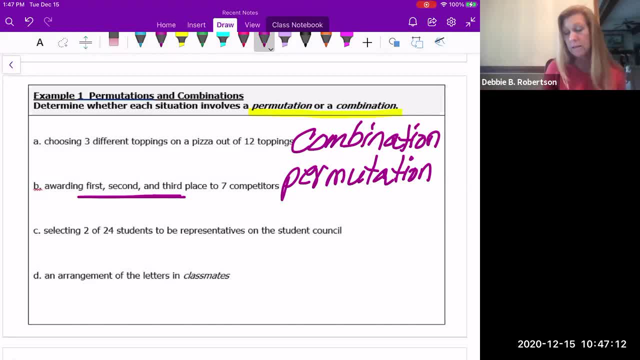 which is when we use the formulas. Using the formula is easy. We just have to know which one to use. All right, What about selecting two out of 24 students to be representatives in student council arena? No, Are you with us? 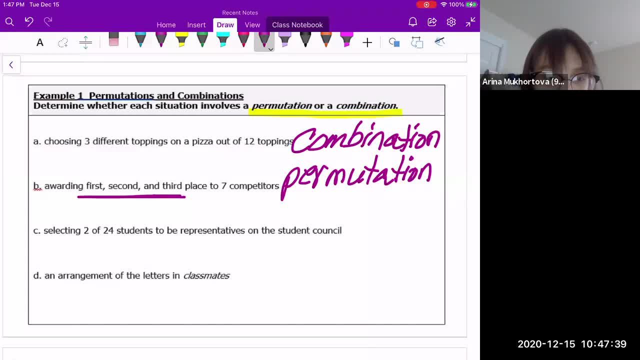 Yes, So combination, Yes, Combination. I'm just picking two out of, say, my homeroom class, All right, And then the last one, an arrangement of the letters in classmates. Yes, Waverly. what do you have to say? 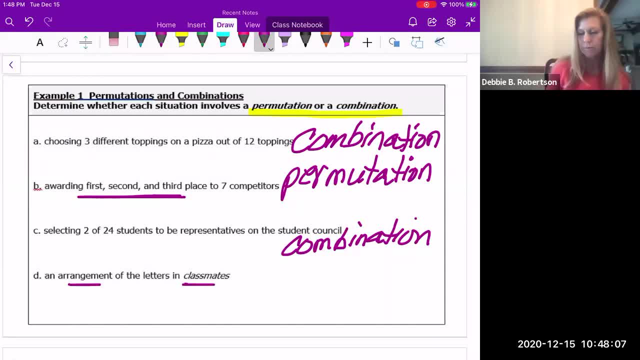 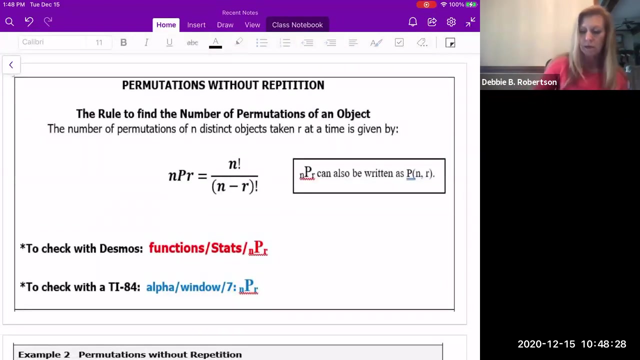 It would be a permutation because it's an arrangement of a particular letters for a word: Yes, All right. So now we've got that part down, how we're going to choose. So let's look at some permutations without repetition. That means, if I pick something, how many ways can I pick this? 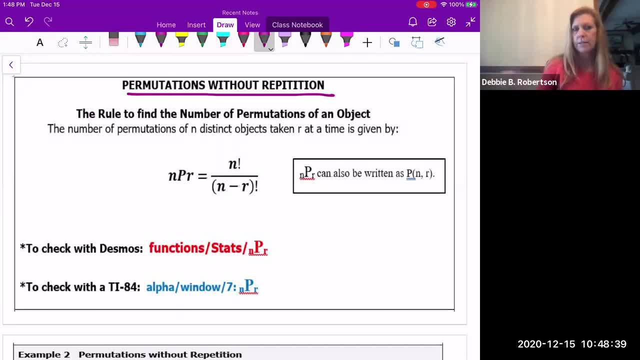 But once I pick one thing, then that's out. you know, no longer an option. All right, So the rule to find the number of permutations that I can have for a particular number of options. So this n represents the number of objects taken are at a time. 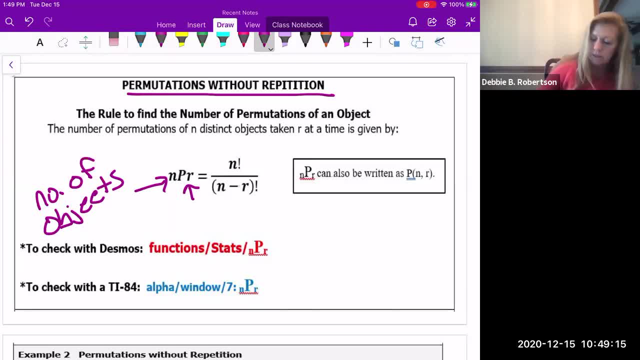 All right. So the number of ways you're going to do it, The number of ways or are at a time Time, I think it's kind of easy to understand, All right. So, in other words, I'm going to pick three things out of 10.. 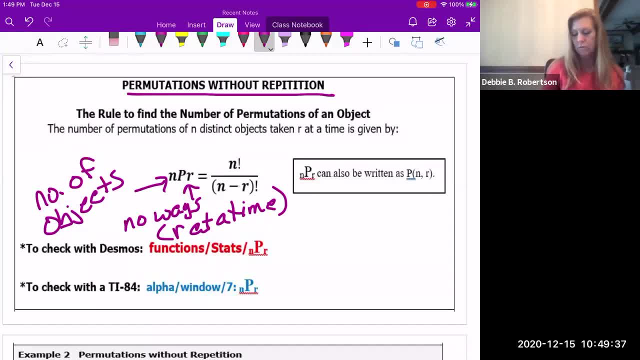 Now this can be. here's the formula: N factorial over N minus R factorial. The NPR can also be written here as P, meaning permutation of N items taken R as a at a time and comma R. When you put NPR in Desmos then you actually enter the data into parentheses like this: 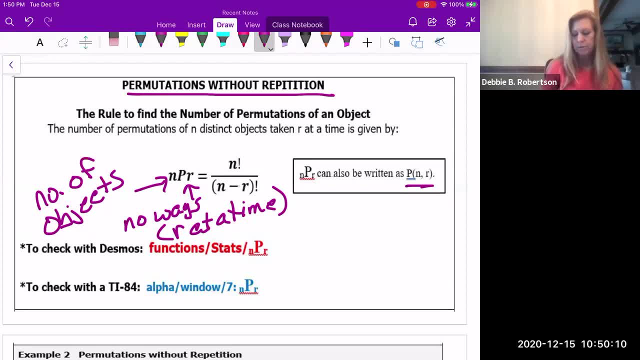 Now I have here to check with Desmos. All right, Here's the keys that you're going to go to. You're going to hit functions, go to stats and choose NPR. I gave you the TI 84. And that is for those who have it. 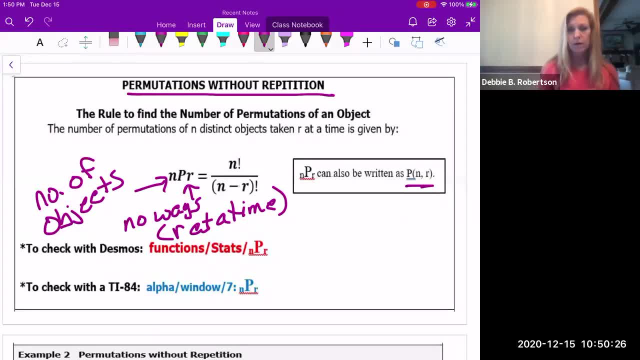 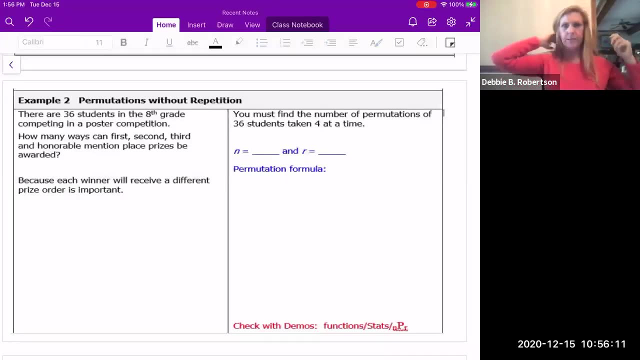 If you don't have one, or might be prepping for an SAT test. there are the keys for that. Okay, So, Okay. So let's look at this example. We have 36 students in eighth grade, So 36 students. 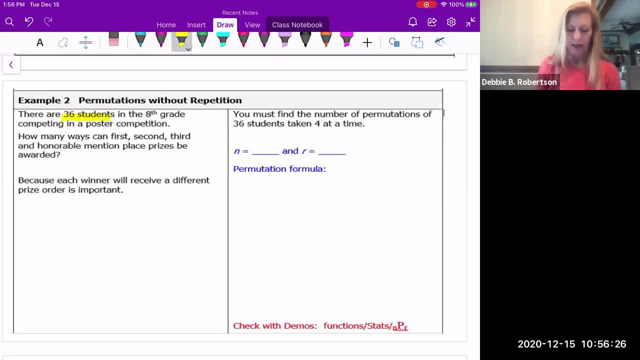 Okay, We have 36 students in eighth grade competing in a poster competition. How many ways can? how many ways can 1st, 2nd, 3rd and honorable mention place prizes be awarded? So how many prizes do we have? 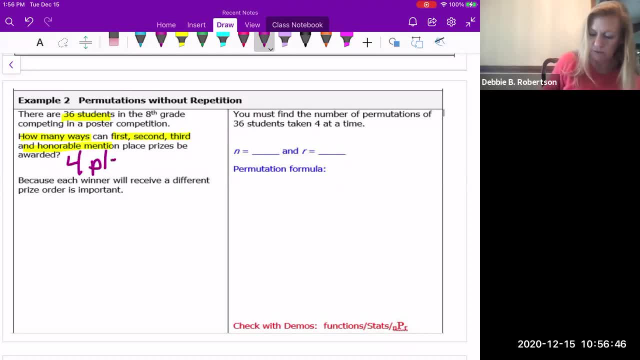 Or place winners. we could say We have four place winners And since we're talking about a poster competition, we're going to say that we have three. Okay, about first, second, third and honorable mention. then order is definitely important. Hence we are. 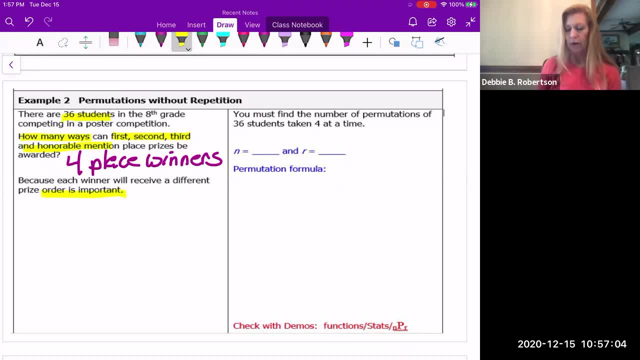 going to have a permutation. So we have to find the number of permutations of 36 students taken four at a time. So 36 students taken four at a time. So what is our permutation formula? Our permutation formula is NPR. okay, equals N factorial divided by N minus R. 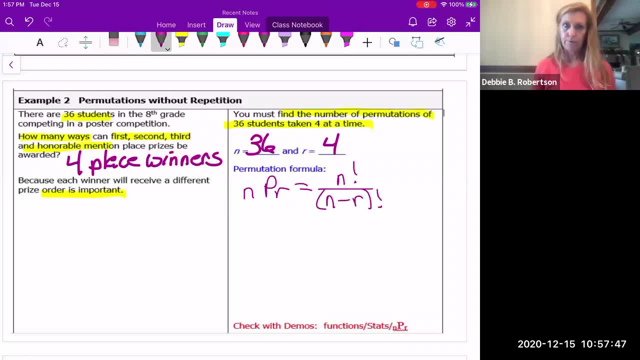 divided by N minus R factorial. So if I substitute in there I'm going to. that means four permutations, taken 36 at a time is equal to 36 factorial divided by 36 minus four factorial. So now I'm going to simplify that. That means 36 factorial. 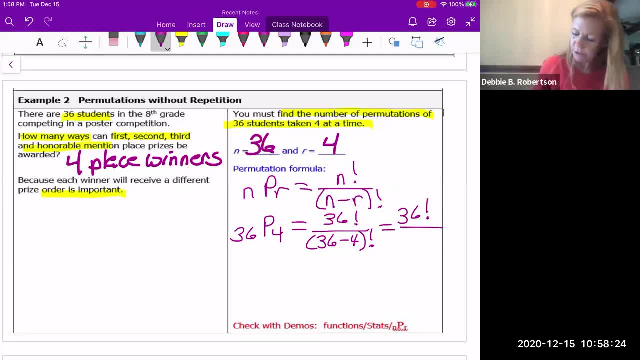 over 36 minus four is 32.. So over 32 factorial. So watch how I can simplify this and divide out my common factors. I could rewrite That fraction as 36 times 35 times five times 34 times 33.. And since I have a 32 factorial, 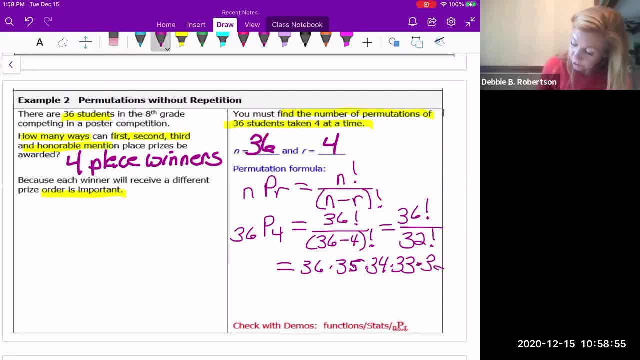 in the denominator I'm going to say times 32 factorial. That's pretty ugly. Let me write that so that there's no misunderstanding: 32 factorial divided by 32 factorial. So the 32 factorials will divide out, And then I can just put the rest into the calculator. 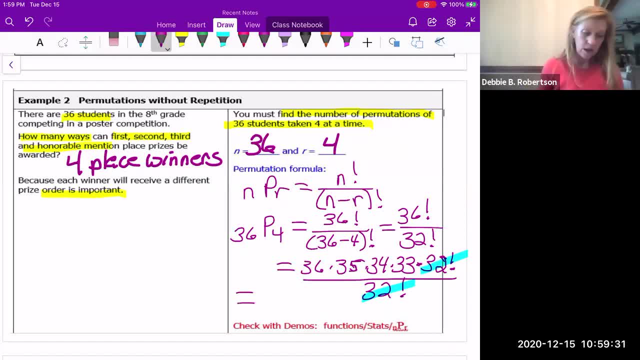 And I end up with 1,413,000.. 1,720.. That is how many different permutations that I have taken, four at a time out of 36.. All right, If I check with Desmos- and I'm going to do this on this one time- 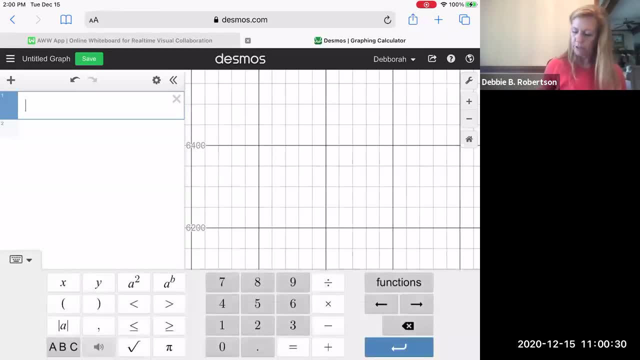 Okay, So I'm in Desmos and I'm going to go to my functions stats and choose NPR, because this is a permutation, and out of 36 comma, taking four at a time, And notice I get 1,413,720.. I may be wrong, not sorMiss. 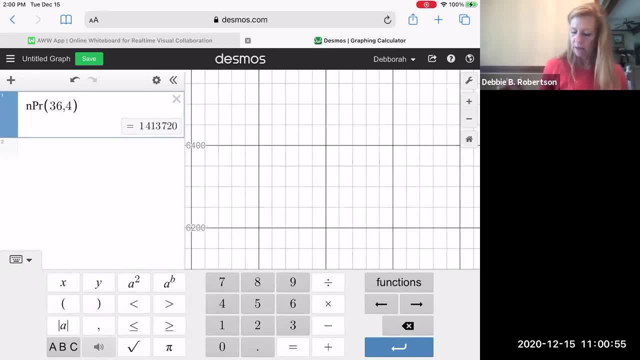 Let me try again toucciolite, But those are only order questions And the hers, so I'm going to tociolit. what they say will determine myН. I've got the same thing that I had when I multiplied what was left. 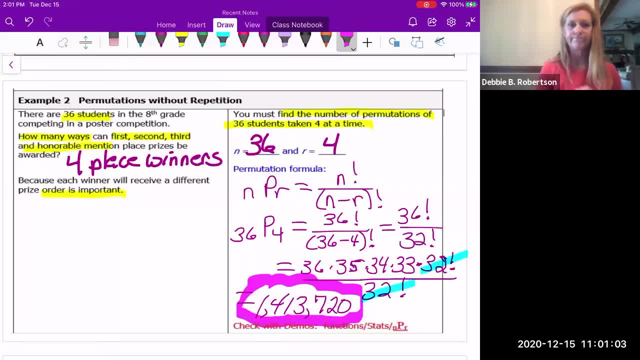 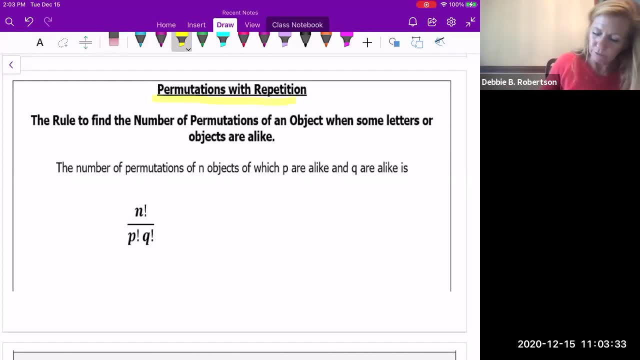 after I simplified that fraction. Okay, So now let's look at permutations with repetition. OK, So now let's look at permutations with repetition. The rule to find the number of permutations of any objects. The rule to find the number of permutations of n objects. 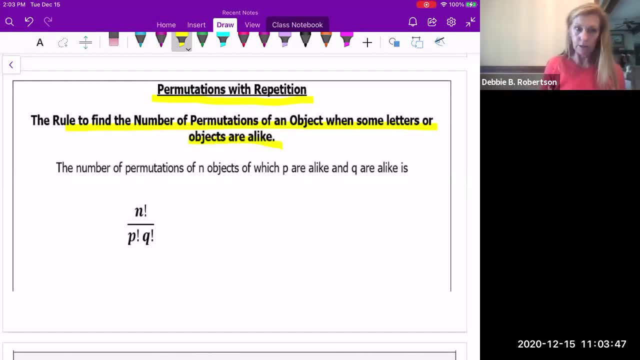 objects are alike, is n factorial over p factorial, q factorial. So let's just say that p and q are alike. So an example of this might be 10 factorial divided by 6 factorial, 3 factorial. It's an example sign, So we could rewrite this. 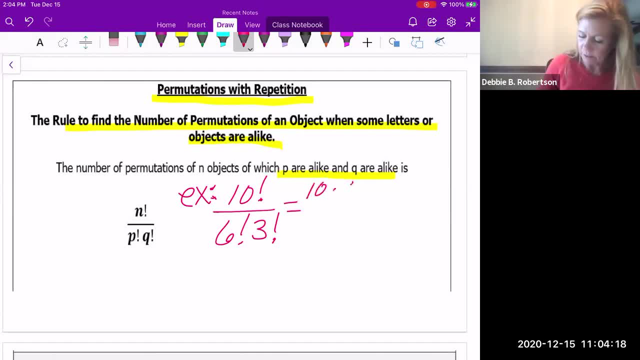 as 10 times 9 times, 8 times 7 times. Since I have a 6 factorial in the denominator, I'm going to say times 6 factorial. Divide that by 6 factorial, times 6 factorial, 3 factorial, And look, I can divide my 6 factorials out and then put in the calculator. 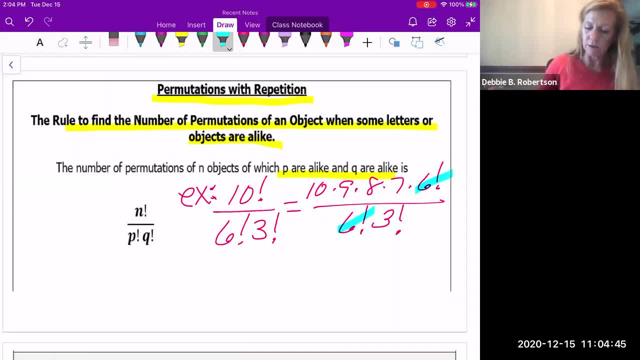 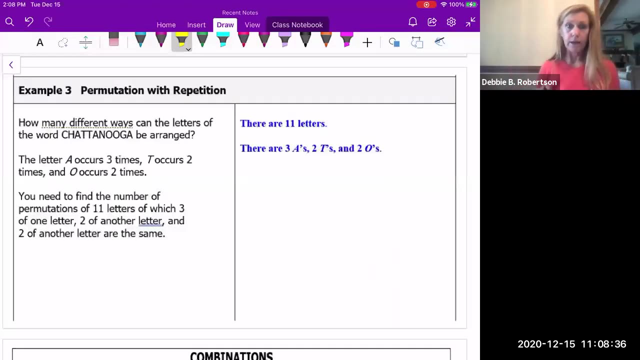 the 10 times 9 times 8 times 7 times either 3 factorial. Hopefully we recognize that that would be 6 at this point, And so our result would be 840.. Okay, so now let's look at permutation with representation. 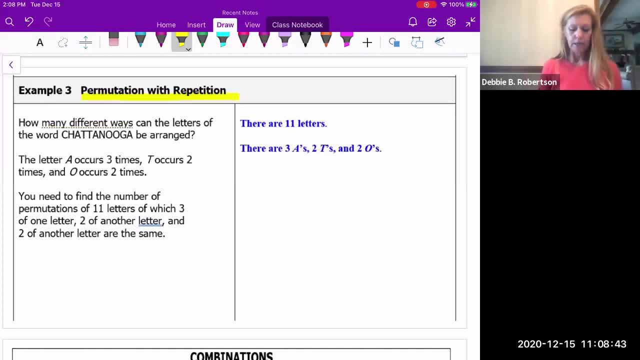 Right. So we want to want to know how many publish ways can the letters of the word Chattanooga be arranged, So ways the letters can be arranged, All right. So notice that in Chattanooga the letter a occurs 3 times and t occurs twice. And O occurs twice. So we need to find that the numbers, okay, that the numbers are well available for a transformation, but only if there's a reason. for example, You don't want anybody that we can't find the quasi equivalent because they always do not know it, That they're even kan ka, the last single expression of an application, Okay. So if you actually fill out this new part of your entries, then you'll see how much you have to read your errors. and all the way up is own the little signs of wills and so on. The way the letters ofR guess n chemical. 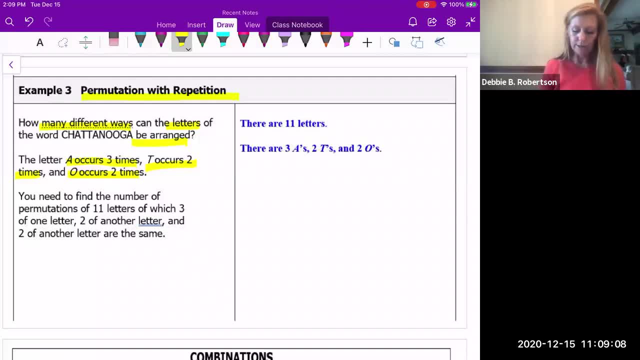 are going to help us in small transitions. So there are k, and a and b are inseparable, But we have to・・・. And O occurs twice. So we need to find the number of permutations of 11 letters, of which three of one letter, two of another letter. 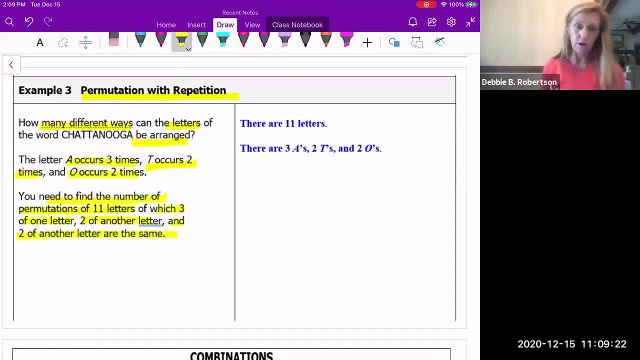 and two of even another letter are the same. Again, there's 11 letters in all, So that means N equals 11.. There we go, All right, And we're going to. since we are having permutation with repetition, some of the letters are the same. 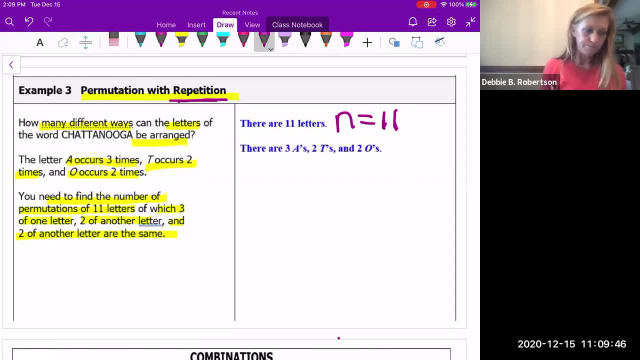 we need to use that formula for a permutation with repetition, And that was N factorial over P factorial, Q factorial. But in this particular case we have we have three different items that are the same, So we're going to have to add an R factorial here. 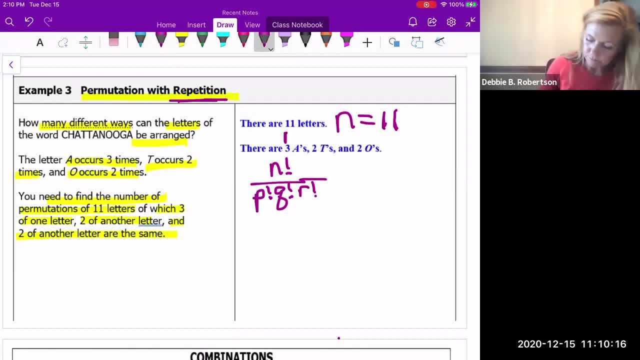 So the A's are going to be our P and the T's will be our Q and the O's will be our R. Now let's substitute: everything in. This is a division sign, So that means we have 11 factorial Divided by three factorial. 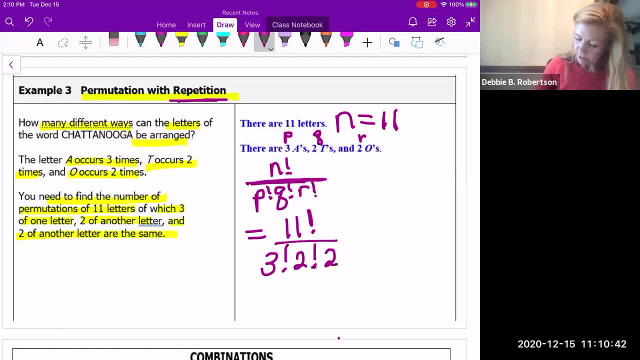 two factorial times, another two factorial. All right, Now we can put all of this into Desmos, And when we do, we will get- let me give myself more room for this- a big number. I'm even going to do it down here. 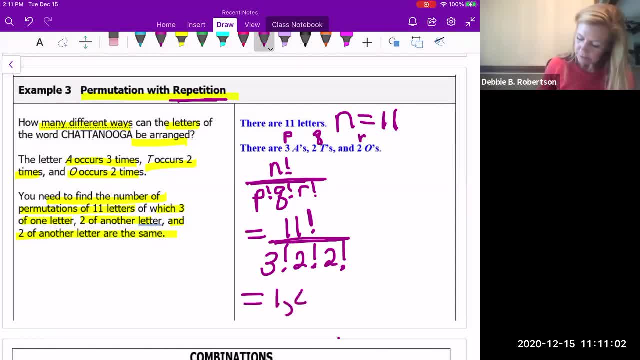 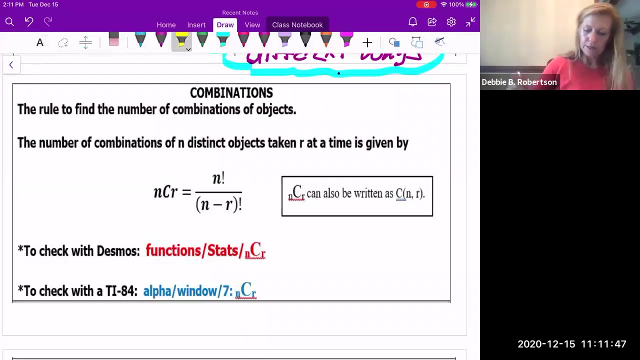 We will get 1,666,000.. 3,200 different ways that these letters can be arranged, Different ways, Okay, Okay, All right. Looking at combinations, the rule to find the number of combinations of objects can be displayed as seen here. 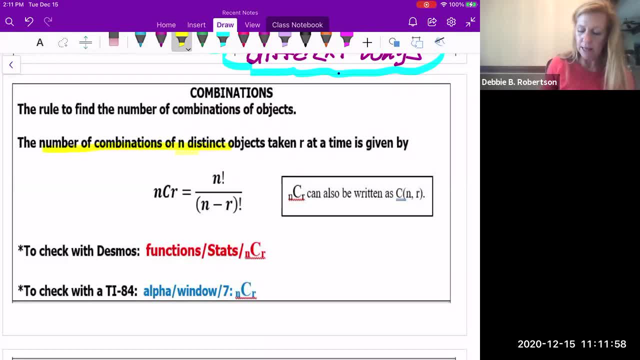 And it is, by the way, the number of combinations of N distinct objects, taken R at a time. Remember that order does not matter for combinations, So our formula is out of a certain number and is the number of objects- Again number of objects- and R is taken R at a time. 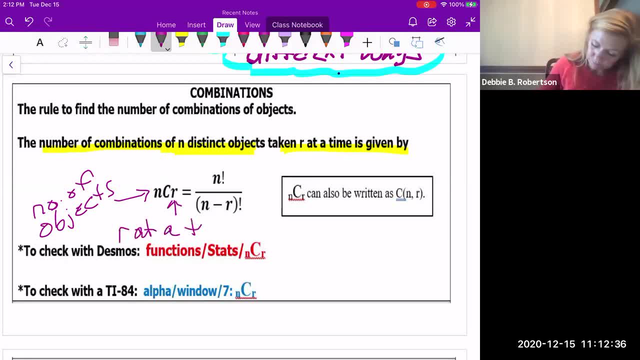 All right. So our formula is N- factorial, So we have N minus R factorial. All right, And in Desmos, once you get there by going function steps NCR, you will, it will open it up as C parentheses And then you will type in your number of objects. 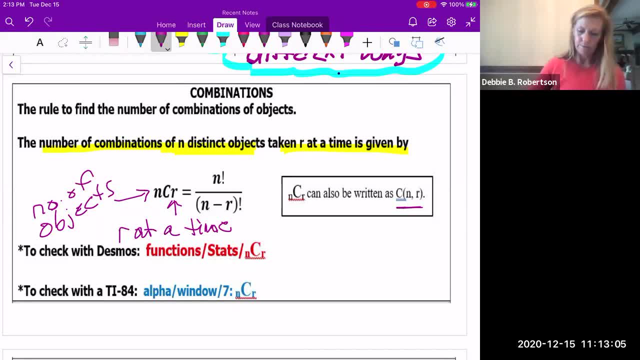 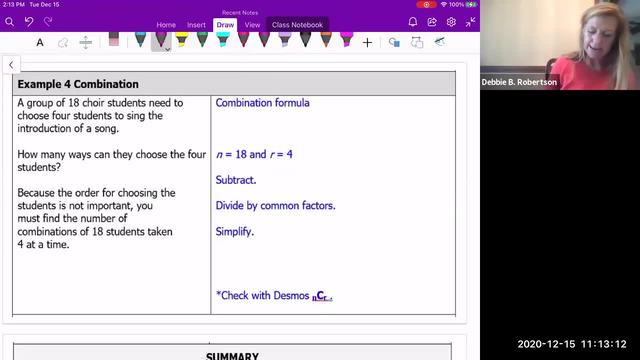 and how many you are taking at a time. So in this example, here we have a group of 18 choir students- oops, 18 choir students. They need to choose four students to sing the introduction song. How many ways can they choose the four students? 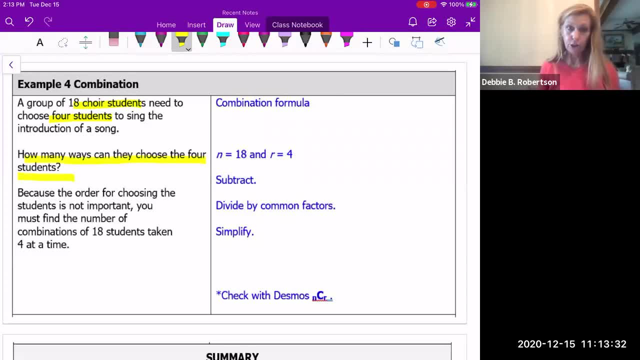 That's what we have to do Now, because the order for choosing the students is not important. I just need to choose four, not a particular one than another one. So the order is not important. That tells me I have a combination. 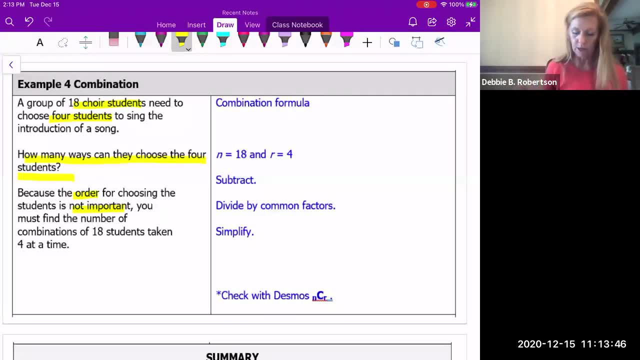 because they don't tell you if it's combination or permutation. It's in the description of the event, that or the situation that we figure that out. But because we do, we have to find the number of combinations of 18 students taken four at a time. 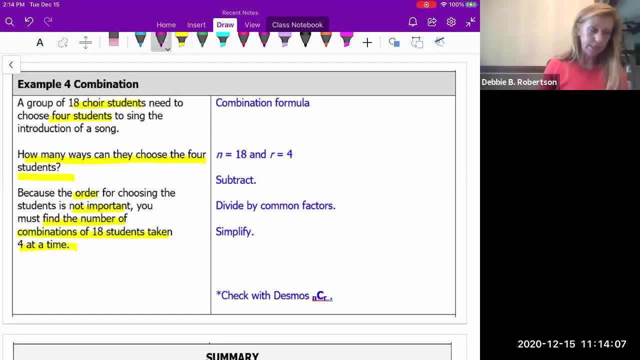 So again, our formula, write down your formula. Your formula is N factorial Divided by N minus R factorial times R factorial. All right, and think about it. If you- if order doesn't matter- you have a lot more opportunities. 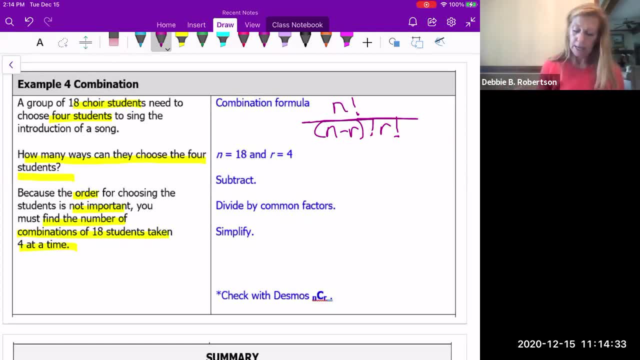 different ways. you could do something All right, and we have it spelled out here that N is 18 and R is four, So we're going to go ahead and substitute N. That means that we have 18 combinations, taken four at a time. 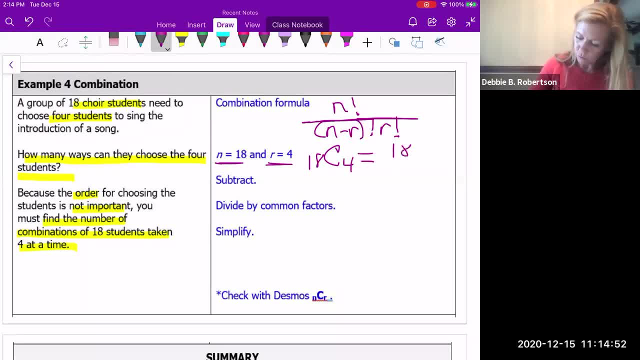 is going to be 18 factorial divided by 18 minus four factorial times four factorial. All right now, if I wanted to simplify that, I would have 18 minus four factorial times four factorial. I would have 18 factorial over 14 factorial times four factorial. 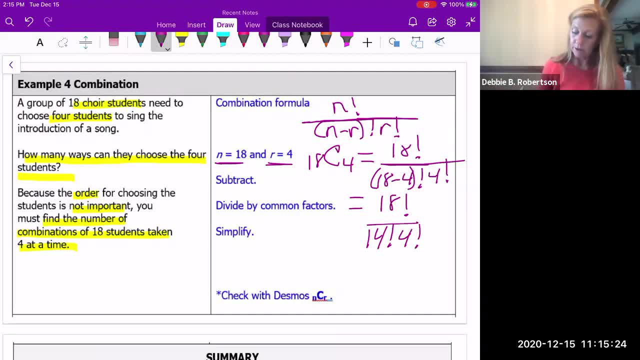 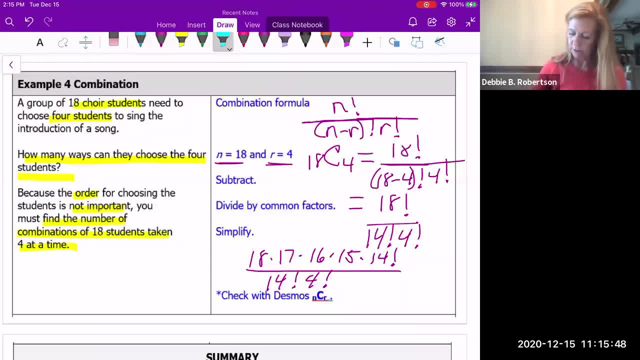 that we learn the math and not just how to put it in the calculator. So the 14 factorials divide out And that is going to leave me with 3,060 ways. Now again, we can put this in Desmos using going to the function stats and choosing NCR. 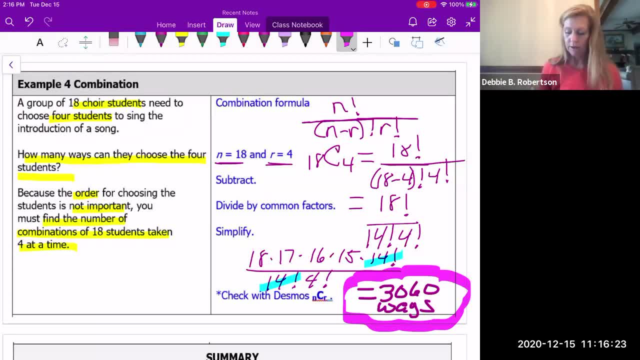 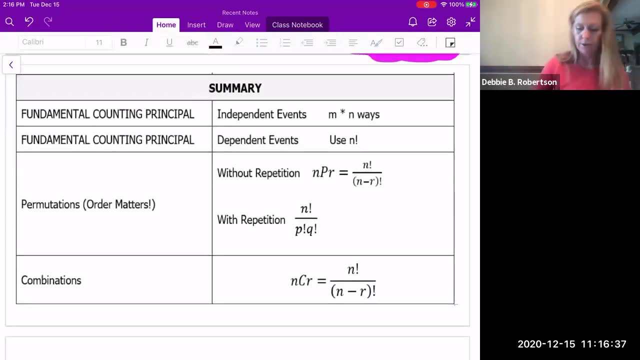 put in your 18 comma four and you will check to see that you have 3,060 ways. So, in summary, here are the things, items we've addressed today. The fundamental counting principle: with independent events we have M times N ways.